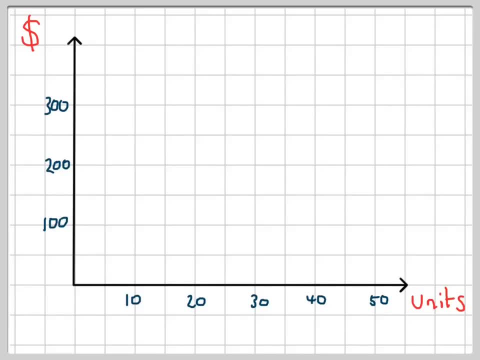 The first thing I'm going to put in is my fixed costs And by their nature, they should stay the same. So it doesn't matter if I sell zero products or if I sell 50 products. my fixed costs will be the same. When we looked at the equation, we said the fixed costs were 100. So if I sold zero, 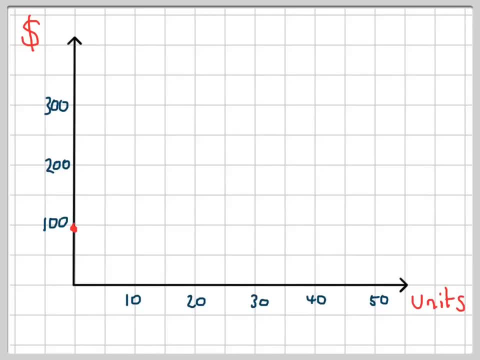 products, my fixed costs would be 100.. If I sold 20, they'd be 100.. If I sold 40, they'd be 100.. And I'm going to end up with a straight line across like this. I've just drawn a better one. 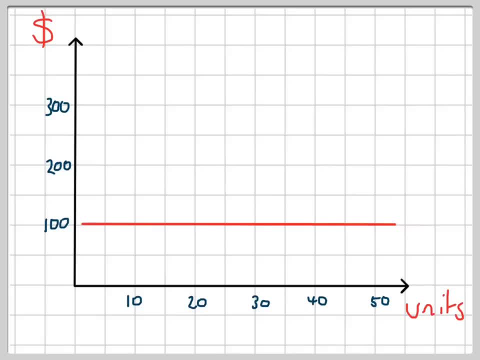 here. Okay, so this line represents my fixed costs. The next thing I'm going to put in is my variable costs, And we said that every product costs 100.. So I'm going to put in my variable costs And we said that every product costs 100.. So I'm going to put in my variable costs And we 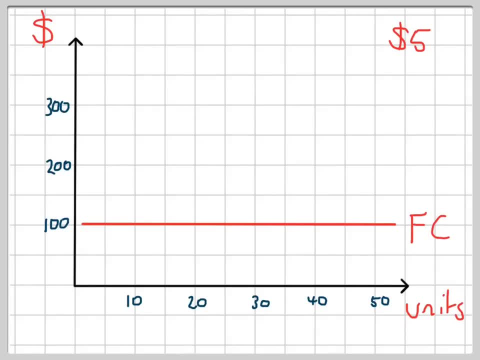 said that every product costs $5 to make. So if I made 10 products, then the cost would be $50.. I'll have a dot here: If I made 20 products, the cost would be 100.. If I made 30, the cost would. be 150, and so on, And I'm going to end up with a straight line like this: And this is my variable costs. The next thing I'm going to put in is my total cost, And total cost is quite obviously just fixed costs plus variable costs. So if I was to sell zero products- so we're down here at zero- 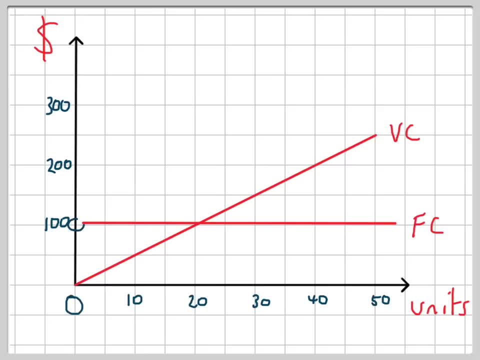 my fixed costs would be 100.. So that's there. My variable costs are zero. So 100 plus zero means that my variable costs are going to start here. When I get to 10, my fixed costs are 100.. My variable costs are 50.. And so at 10, my total costs. 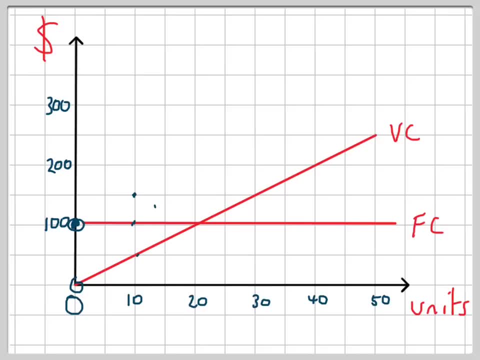 are going to be 150.. For 20 units, you can see here that both my fixed costs and my variable costs are both equal to 100. So my total costs are going to be equal to 200. And if I keep on going like that, I'm going to end up with 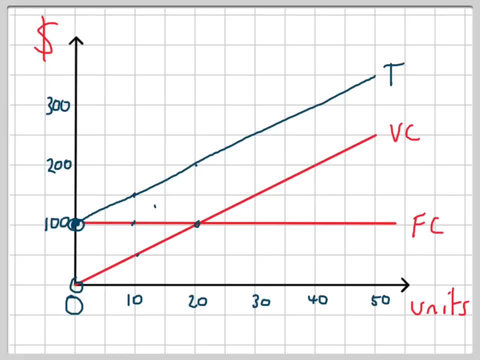 a straight line like this: This is my total cost. Now, my total cost is always parallel to my vertical costs And if I keep on going like that, I'm going to end up with a straight line like this And just shift it up by the amount of the fixed costs. So if I take 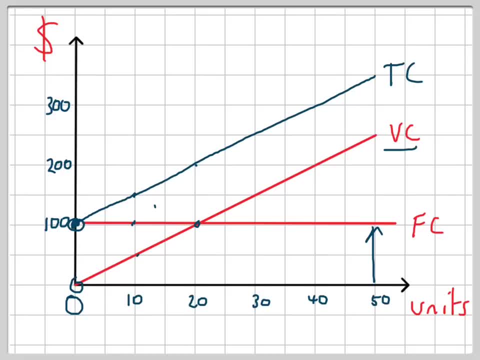 these fixed costs. I've moved it up two lines You can see here. so this is one, two lines, that I've moved my fixed costs up. So this variable cost is going to just be parallel but moved up one, two lines all the way along One, two lines. So it's parallel to variable costs. 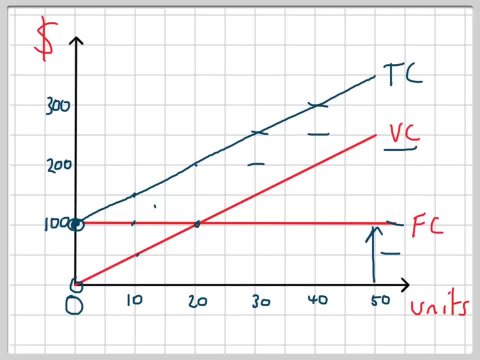 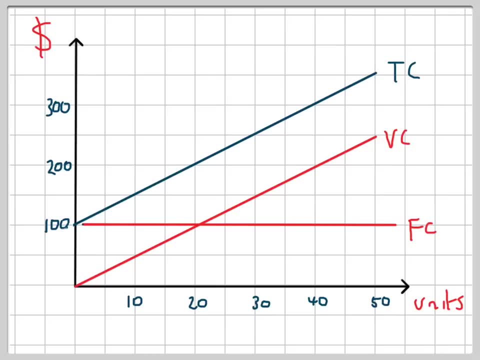 moved up by the amount of the fixed costs. Okay, so that's what it looks like so far. There's just one more line that I need to draw in, and this is revenue, And the revenue is: how much money do I receive from the products that I sell, If I sell? 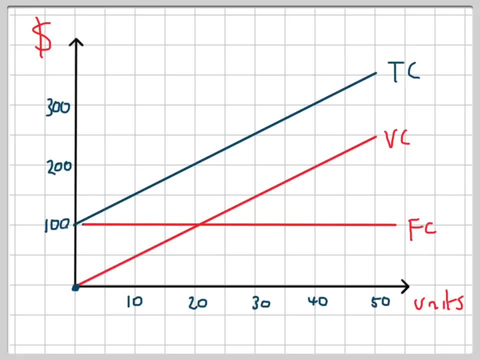 zero products, I make zero revenue. If- and remember- I was selling the products for $10 each. If I sold 10 products, I'd make $100 in revenue. If I sold 20 products, I'd make $200 in revenue. 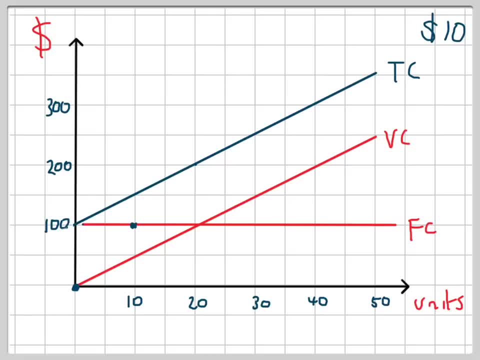 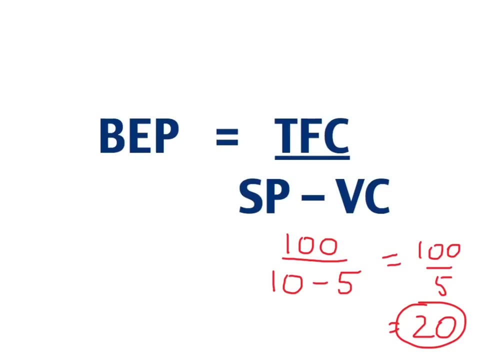 If I made 30 products, I'd make $300 in revenue, And so I'll end up with a straight line that looks like this, which I call revenue. If I went back to my equation, we said that for this example, that for $100 of revenue of fixed costs divided by the selling price minus variable, 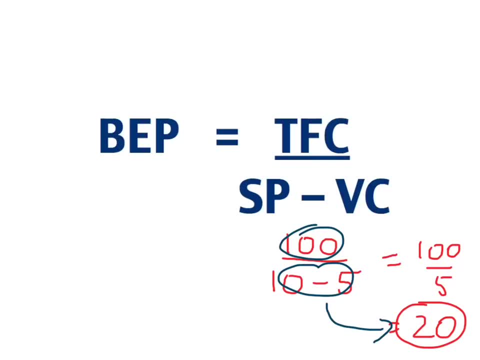 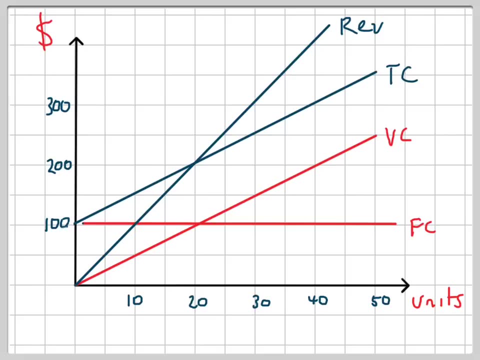 costs. I would need to sell 20 units in order to break even. Now my graph shows me, for the same example, exactly the same thing. The break even point on this graph is where revenue equals total costs, So the total amount that I'm spending. 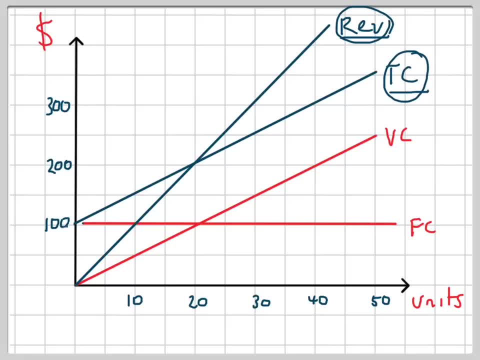 is the same as the total amount that I'm receiving, And you can see that that happens here. That's where revenue equals total costs, and that's at 20 units, which is exactly the same as what the equation said, which is what should. 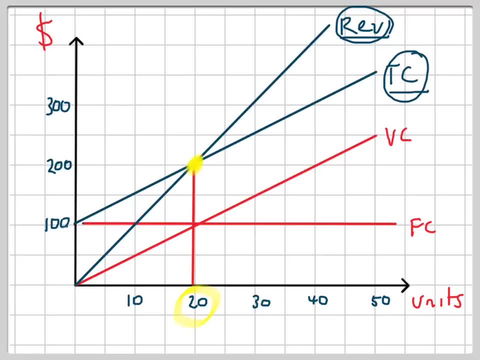 happen every time. So the equation and the graph should show exactly the same information. You can see that if I only sold 10 units, then there's a gap here where total costs- the line on the top- is greater than revenue, which means I'm spending more money than I'm.